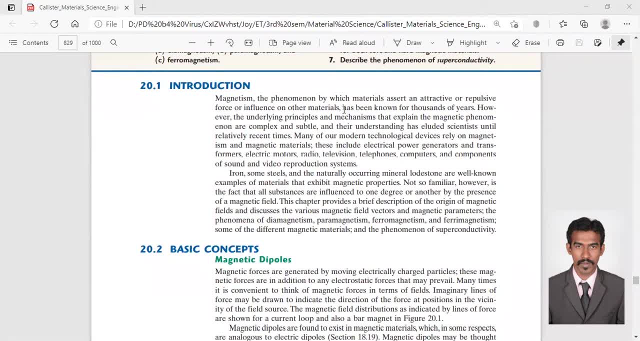 principles and mechanisms that explain the magnetic phenomenon are complex and subtle and their understanding has eluded scientists until relatively recent times. So the phenomenon behind that, how only some materials are attracting, why some are not attracting. So these kind of phenomena still under discussion. Many of our modern technological devices rely 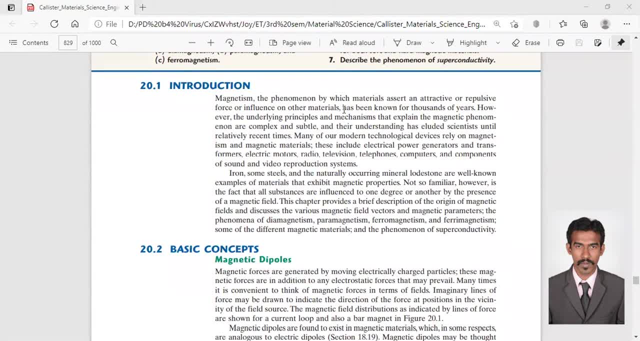 on magnetism and magnetic materials. These include electrical power generators, transformers, motors, radio, television, telephones, computers. So these all are dependent on the magnetism. you know, right, Motors, they need temporary magnet. right, Electromagnet Telephones. 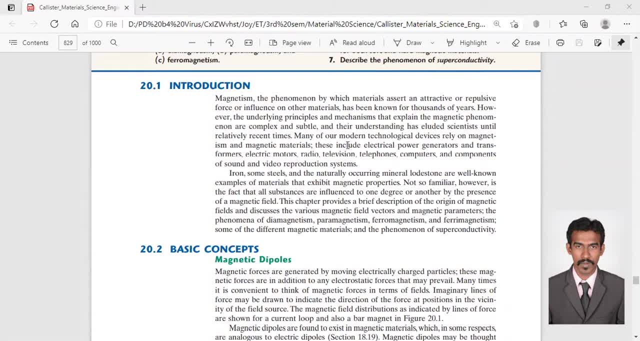 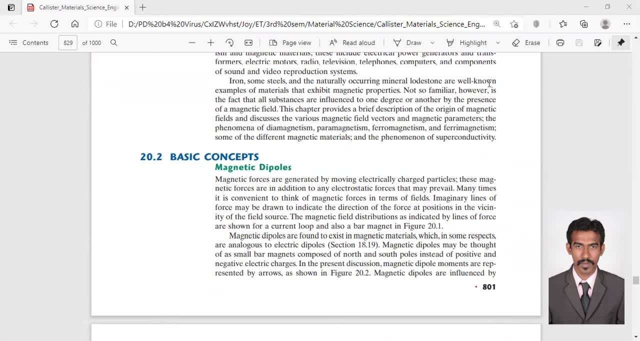 right. So these all need this magnetic property Right? Iron, some steels and the naturally occurring mineral lodestone are well-known examples of materials that exhibit magnetic properties. So you know iron and some steels. usually they exhibit magnetic property. Not so familiar, however, is that the fact that 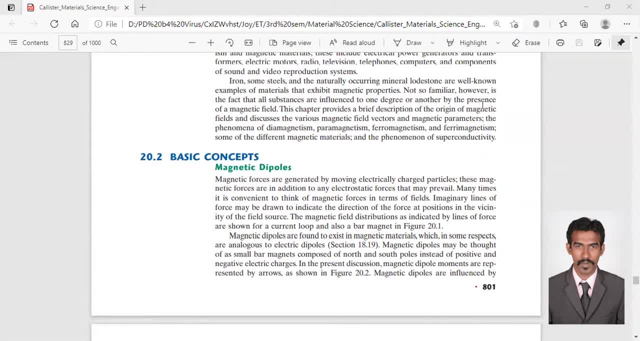 all substances are influenced to one degree or another by the presence of magnetic field. So, this presence of magnetic field, there are chances that they are getting magnetic attraction, So this is a phenomenon. So this is a phenomenon. So this is a phenomenon. 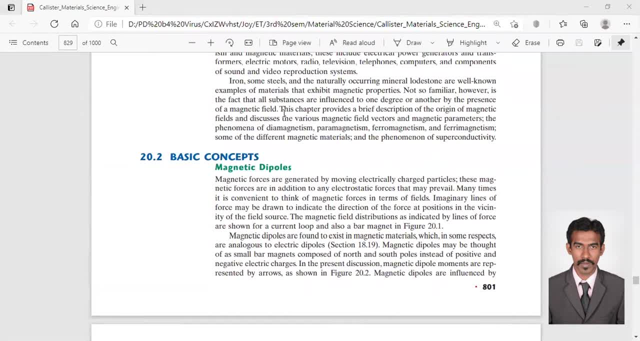 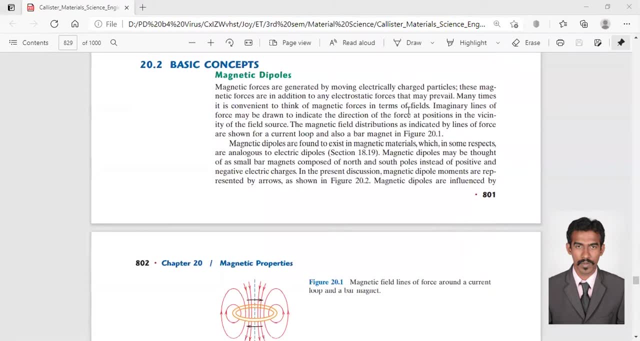 But the strength is different. The strength is varied. So this chapter provides a brief description of the origin of magnetic field and all about the magnetic field. So we'll see Basic concept: Magnetic dipoles- right, Magnetic dipoles. Magnetic dipoles are generated. 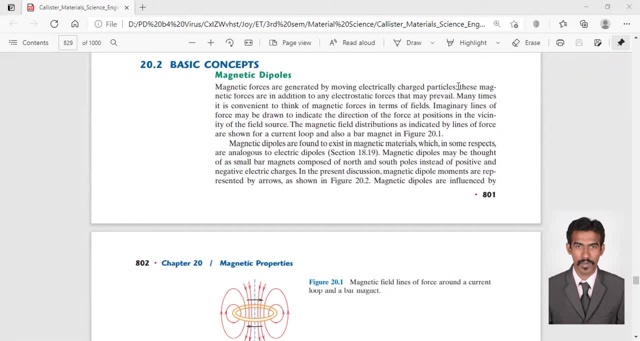 by moving electrically charged particles, right? So you know, usually magnetic fields are generated by moving an electric field. So you know, usually magnetic fields are generated by moving an electro- I mean charged particle- through a current flux, right, Or electric flux. These 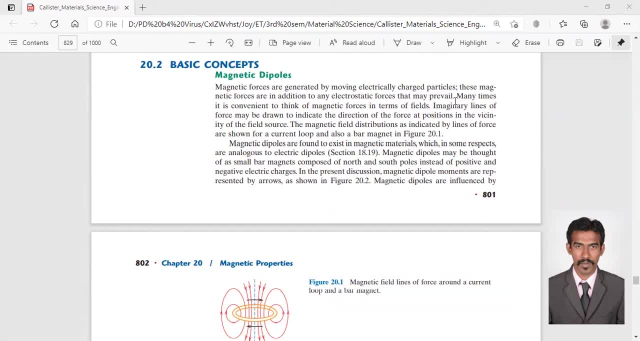 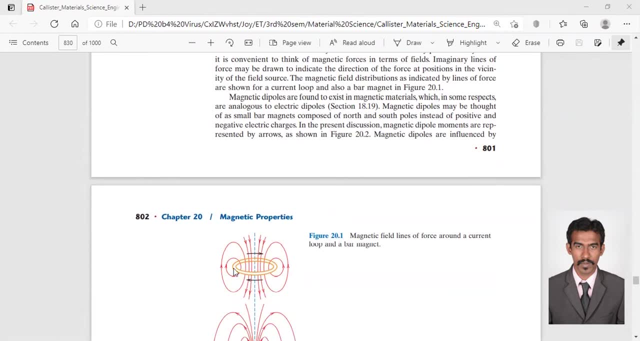 magnetic forces are in addition to any electrostatic forces that may prevail. Many times it is convenient to think of magnetic forces in terms of fields, right? So magnetic field? usually we call it as magnetic field. You see, So these are magnetic fields. Imaginary lines of force may be. 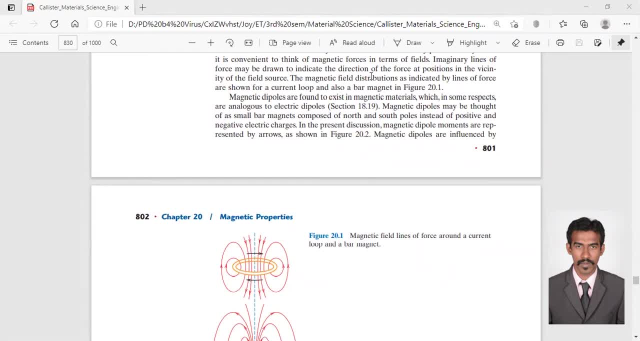 drawn to indicate the direction of the magnetic field. So this is a phenomenon, So this is a characteristic history that characterizes magnetic field and any reaction of the force. So magnetic dipoles are found to exist in magnetic materials which in some respects are: 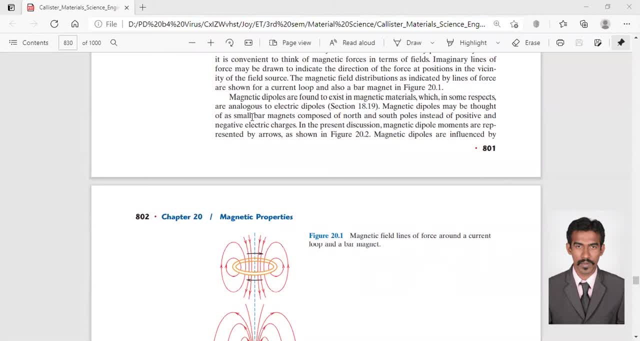 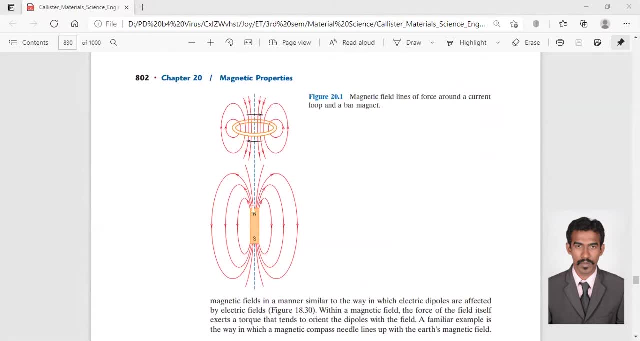 analogous to electric dipoles. So when you see here, yeah, this diagram, so this, usually you know right, The magnetic field activity from north to south, So field lines start from north and will end up in south, right, But if you look here, this is a�† new sign in the objective тому. this is another. 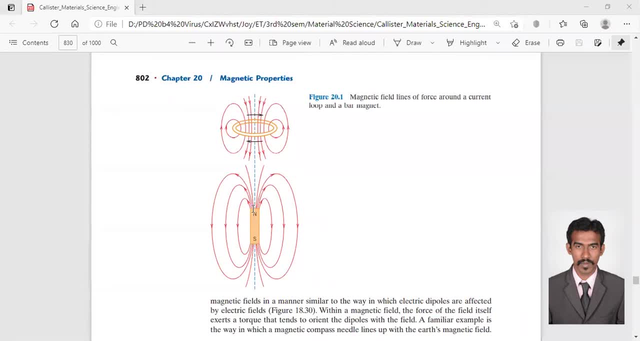 group of dichrom Uberian into Civilization. So these are not the zitten, But there are other types ofousing in the în artist art filter and Racing back to times. I'm not talking about dynamic tools, so they will go like this all the way around and ended up in here, right? so this is a magnetic field. 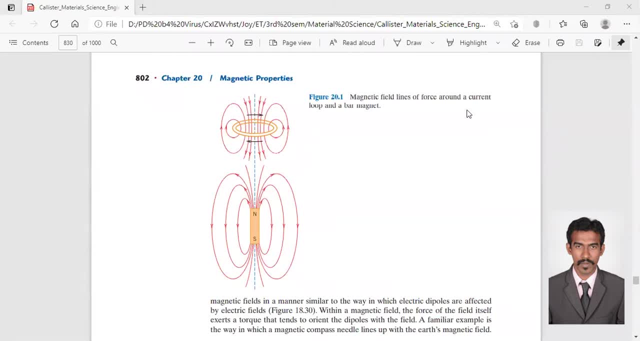 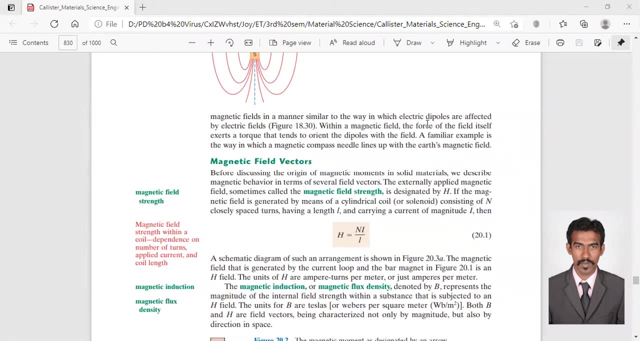 lines, magnetic field, lines of force around around loop and bar magnet- right, so this is bar magnet and this is current loop. okay, right. magnetic fields in a manner similar to the way in which electric dipoles are affected by electric fields within a magnetic field: the force of the field: 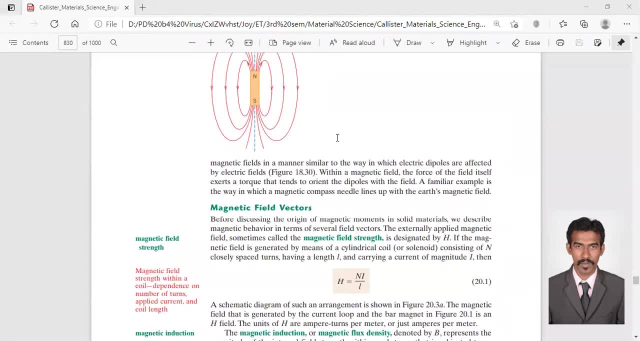 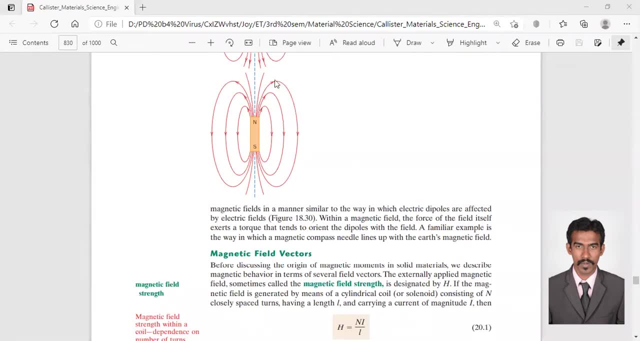 itself exerts a torque that tends to orient the dipoles with the field right. so if you have a material that will tend to insert a toe on this direction- a familiar example is the way in which a magnetic compass needle lines up with the earth's magnetic field. so if there is an already available 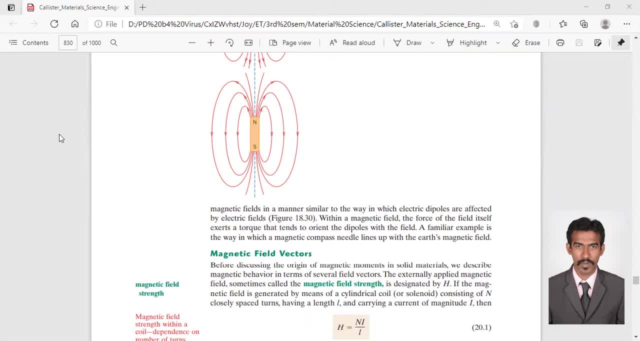 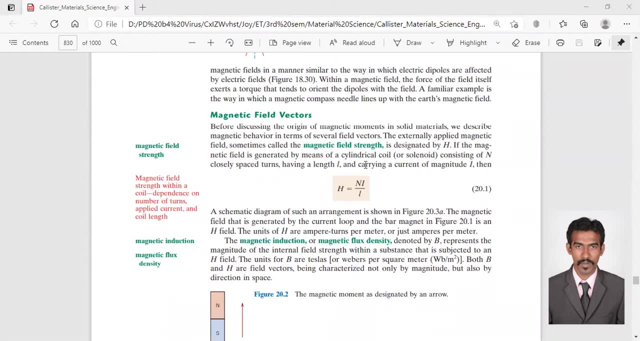 magnetic field, which is earth magnetic field. you know the compass will also take that particular direction: magnetic field vectors. so we will discuss this formula. first time we describe behavior in terms of several field vectors. the externally applied magnetic field, you sometimes called as magnetic field strength. that is this edge right. so edge the magnetic field. 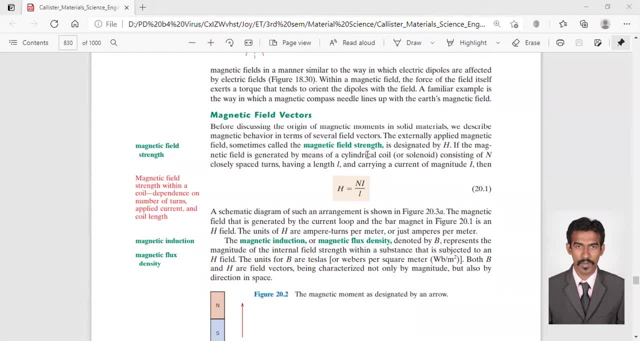 strength if the magnetic field is generated by means of a cylindrical coil or solenoid. right? so you know what is the solenoid? is you know? it is something like this. okay, this is what called as a solenoid. all right, cylindrical coil of solenoid consisting of n. 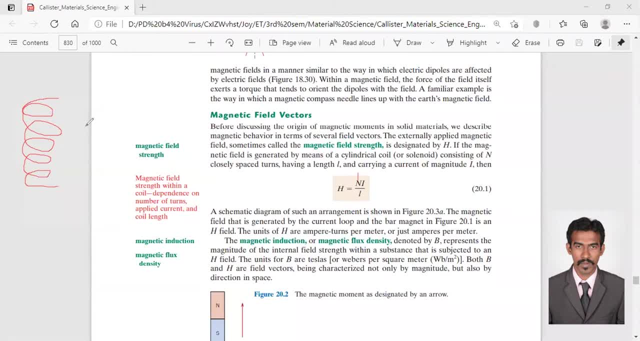 closely spaced turns. so this n is the number of turns here: one, two, three, four, five, like this right number of turns across these much turns having a length L. so this length is the L right, this length is the L, and carrying a current of magnitude, I right. so this 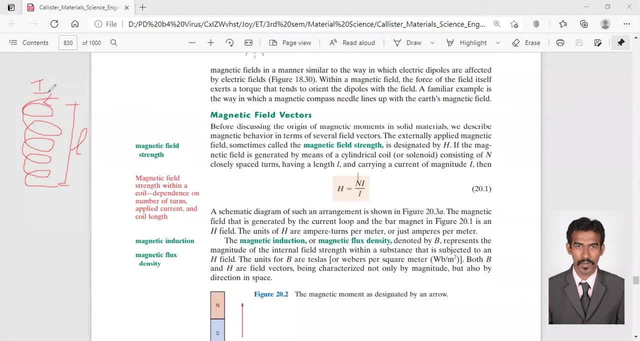 conductor should have carrying a magnitude of I current right, then a schematic diagram of such an arrangement is shown in the figure at twenty point three A. so magnetic field acts with small n and by sort of Mercille engines. so this is what you get. so actually, as long as your Checkpoint X is, 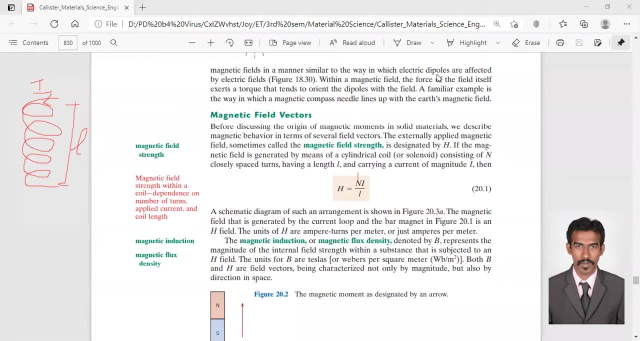 seeing this with this form there. then you just have to insert the pointer ticket over here- positions here, which then creates the. the zip that I have left over in the D sigma column related to the velocity is basically Butterfield Cit线. So the reason I go to that drawing: yeah, here we have that right. 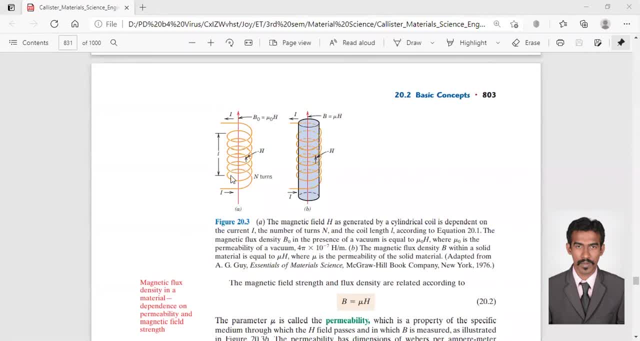 So this is what called as the solenoid, okay, which is carrying a current of. I right This, I is passing through this and coming out by this way, And the length of the solenoid is given as L right. 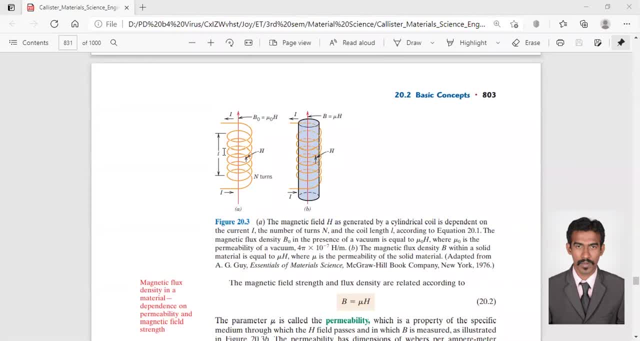 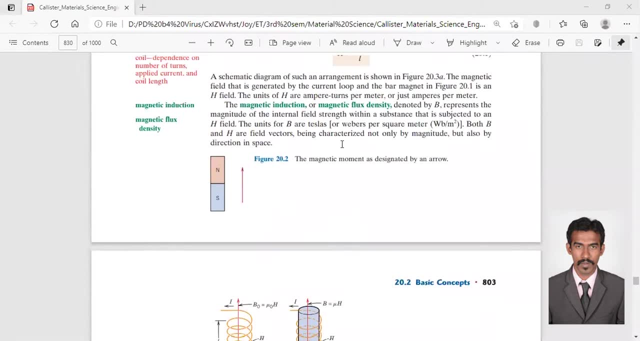 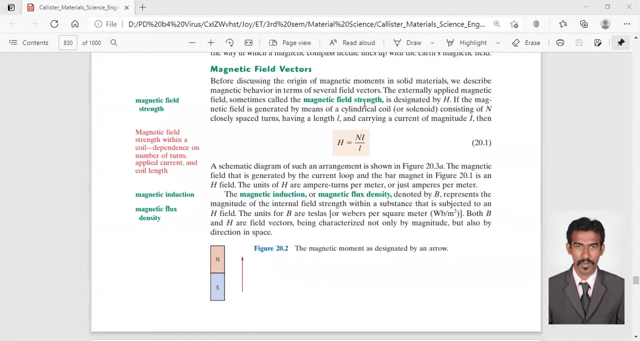 Then length of the solenoid is given as L, So the magnetic flux generated, it is H, right When you put this in the formula. H is equal to N into I, into N, I upon L, right. So the magnetic field strength, H is equal to N, that is number of coils, into I. that is current, the magnitude of the current divided by L, that is length of the conductor. right length of the conductor. 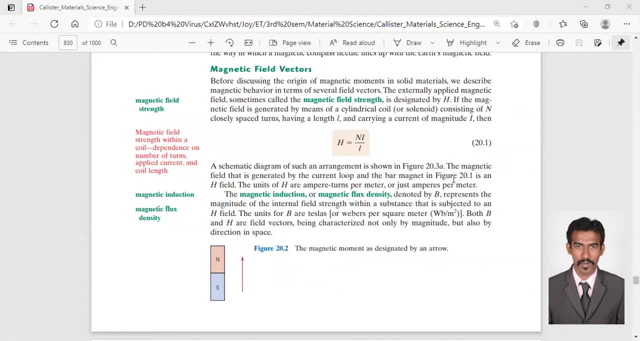 The magnetic field that is generated by the current loop and the bar magnet is an H field. So here the Field is H. The unit of H are ampere turns per minute, sort of per meter. Ampere I is ampere, N is turns per length. is given in meter right. So unit is simple: Ampere I is given in ampere, turn is given, N is given in turns and L is meter. So the unit is ampere turns per meter Or just amperes per meter. So all these things. 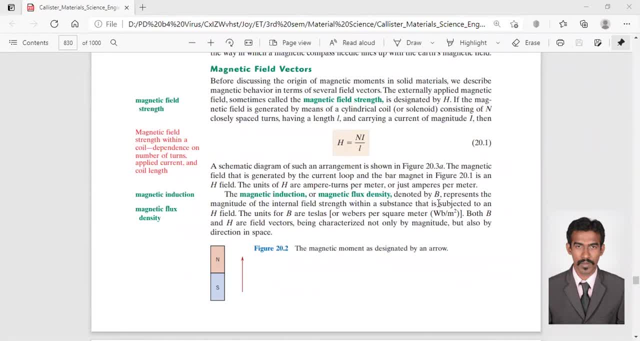 When we look at the journalists'atalog holdings where arbitrage isuxe, what we observe to do is that in the linguistic, I really anxiety very much. I found something too. No First, please, Yeah, Round it, Bye, Bye. 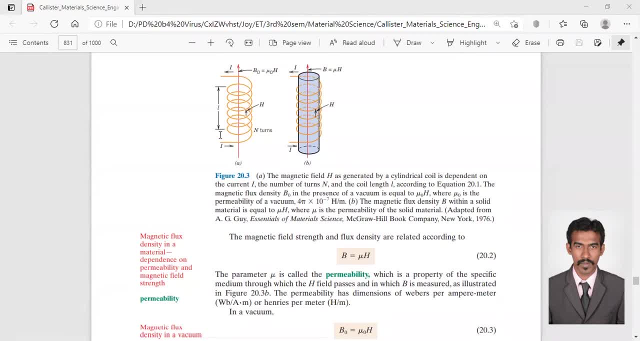 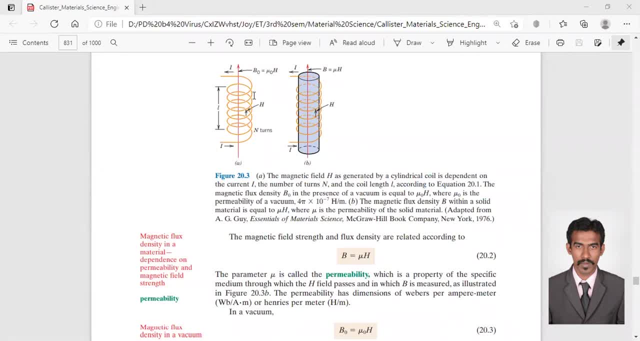 much is the current passing through is a dependent factor. a number of turns in right, so number of turns. so when the turn increases the magnetic field strength increases. right, when the current increases, the strength increases and with the coil length that will decrease the magnetic flux density. d? naught is the presence of vacuum. is equal to mu? naught into h? yeah, me not. is the? 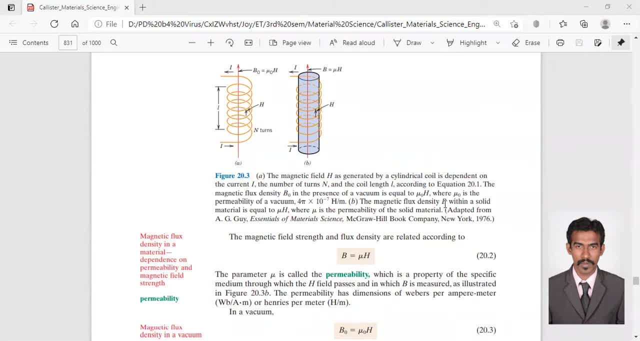 permeability of the vacuum magnetic flux density b, e within a solid material is equal to mu h. yeah, mu is the permeability of the solid material and mu naught within the vacuum. right, there's a wave, not just you know. yeah, yeah, this mu naught is the permeability in. 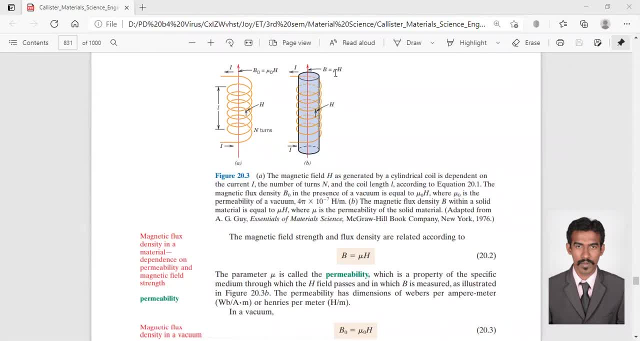 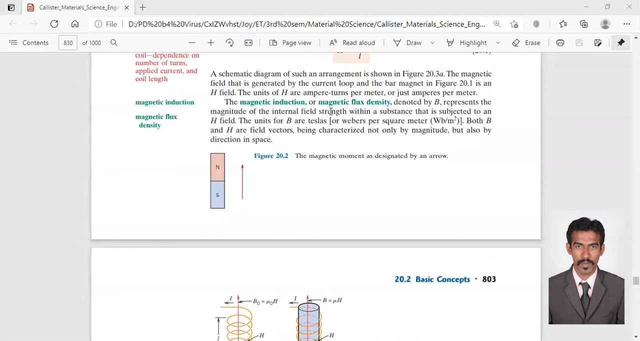 the vacuum. so this equation is for field strength within the material right. within the material, this h is created due to the current passing around the material right. that's the difference. so here this d represent the magnitude of the magnetic field that is given by theyon side and d is the magnetic field strength. 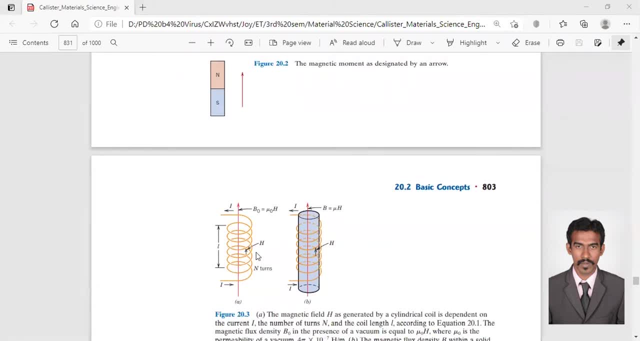 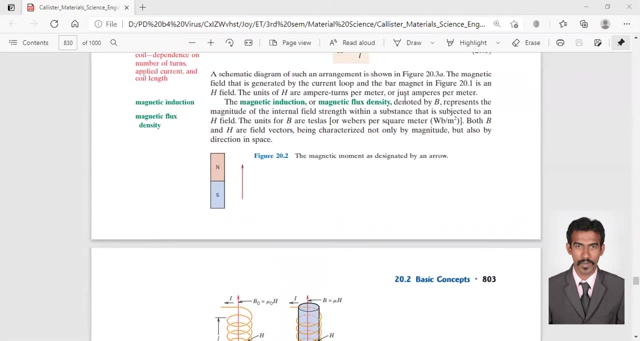 this h is created due to the internal field strength within a substance that is subjected to an edge field right. so if it is subjected to a magnetic field h, the internal field is given by b. right internal field is given by b. uh, the unit of b is tesla or weber's first square meter right. 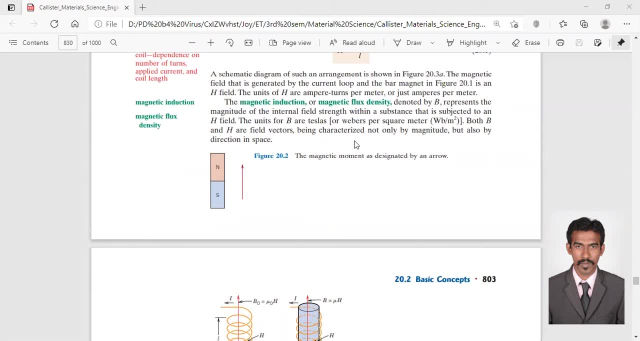 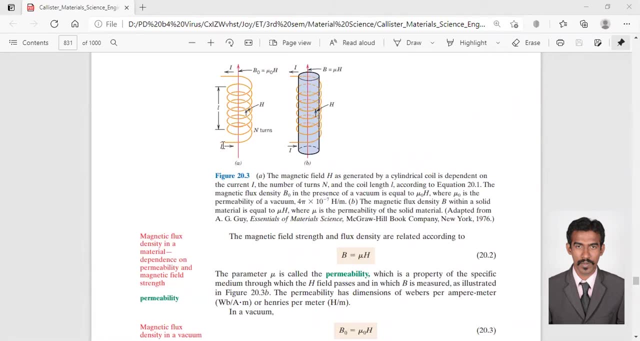 we'll either put it as like t capital, or wb per meter square, are field vectors being characterized not only by magnitude but also by direction in space, right? so when you see, everything has a direction. so current is going by this way, coming by that way, field strength is going that way, right, this is going this way, so everything. 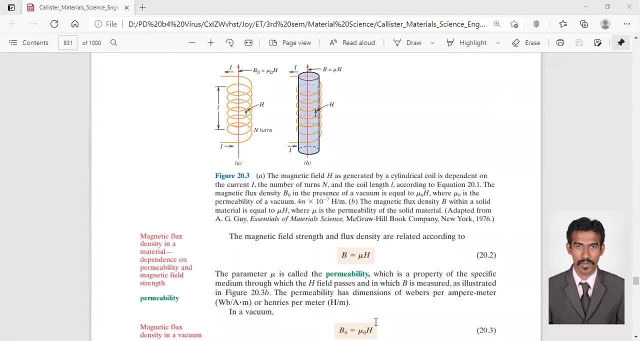 has a direction. right, everything has a direction. magnetic flux density: be right, this is magnetic flux density b and this is magnetic field edge. two are different things. within a solid material is equal to mu into h, so b is equal to mu into h. right b is equal to mu into h. 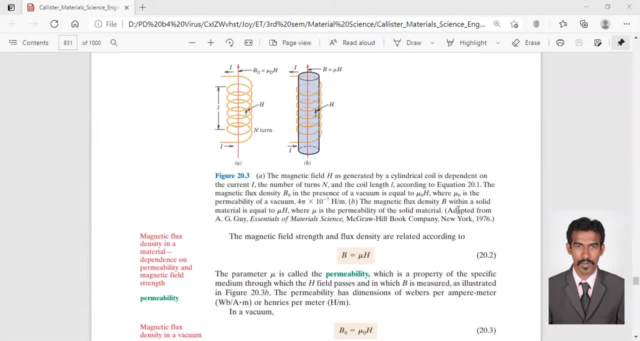 where we will see what is this mu is right. b is the represents of a presence in a value. vacuum is equal to mu naught. h right. so this mu is a variable. if it is vacuum, it will take mu naught. if it is some other material, that will take mu which is a value right where mu naught is a. 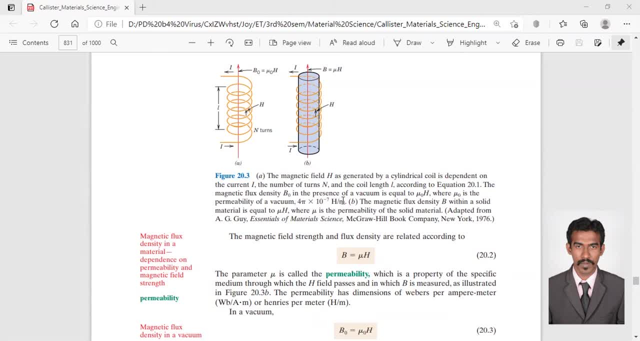 permeability of a vacuum, that is 4 pi into the power minus 7 h per m. right to the power minus 7. you see the value right. flux density b within a solid material- right. so now it's not vacuum, it's a solid material- is equal to mu h. right, that is mu h, where mu is permeability of the solid material. 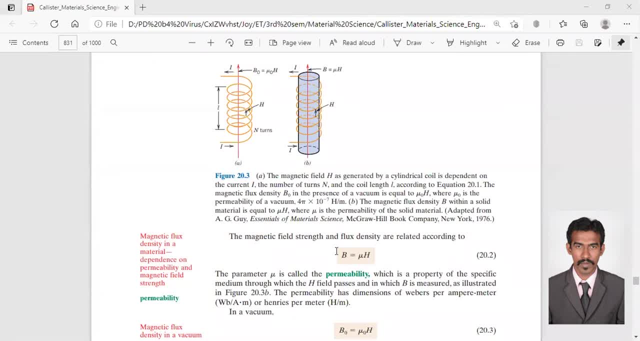 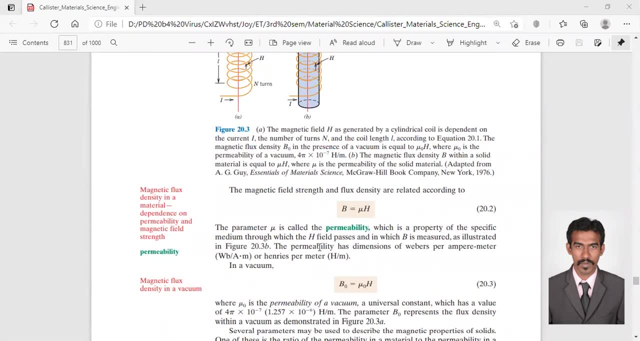 right. so here the mu is the permeability of the solid material. so parameter mu is called as the permeability, which is a property of specific medium through which the h field passes and in which b is measured, all illustrated in this figure, right. so here permeability is the property of specific. 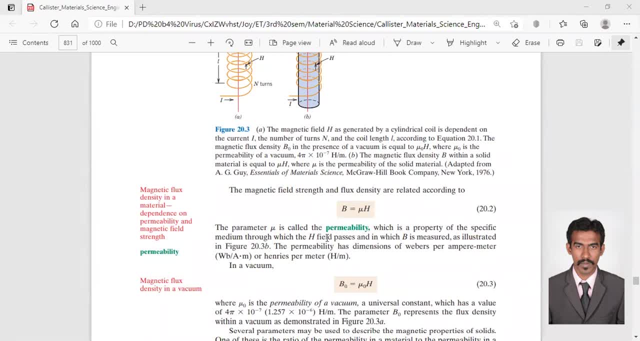 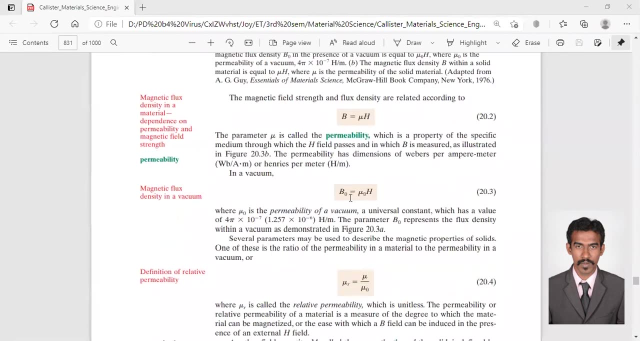 medium through which the h field passes. so to pass these fields need a medium and in which b is measured right. the permeability has dimension of weber's per mta meter, that is wb per am or henry's per meter hm. also we can say in the same case: while in vacuum, that is, b naught is equal to mu. 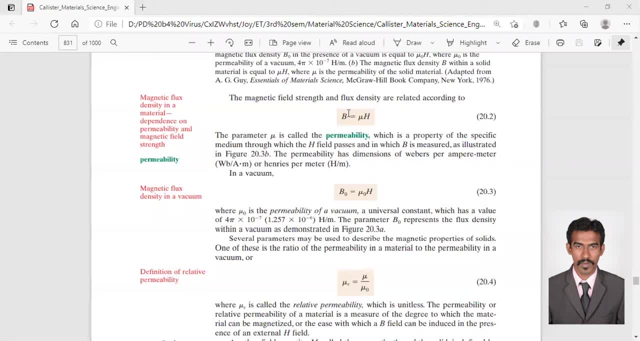 naught into h. same equation: if it is a solid material that will take, b is equal to mu h. when in a vacuum that is b 0, v naught is equal to mu naught into h, right, we are not into h. where mu naught is the permeability of the vacuum and inverse and constant. 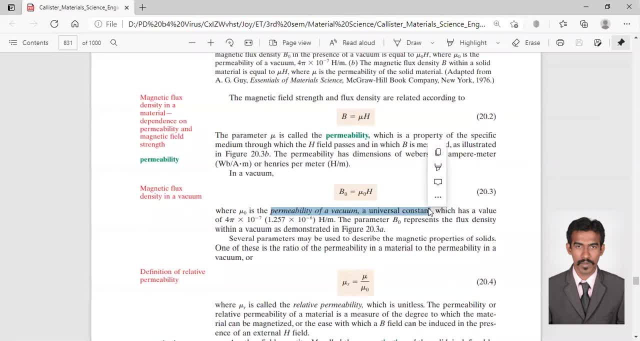 right, so this one is a universal constant which has a value of 4.0 minus 7. okay, so this is the terms related to magnetic flux density and magnetic field strength.